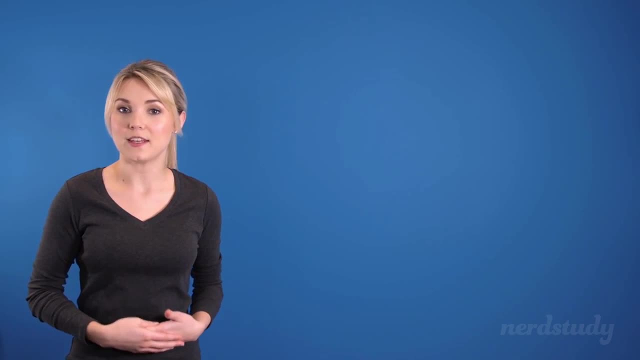 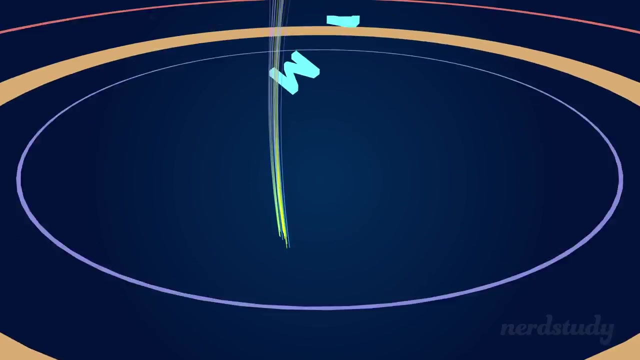 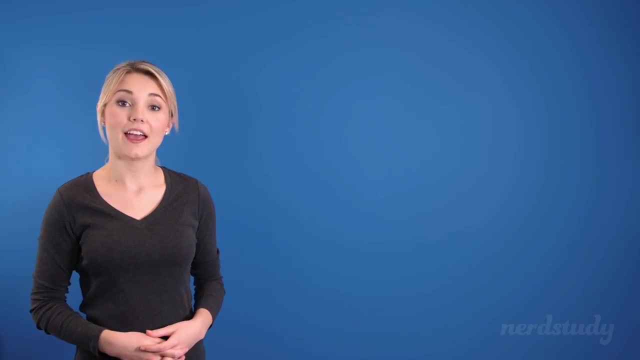 So we've already talked a bit about sequences, but now we're going to actually put some more specific terminology to them and look at them in a more general sense. So in this video, let's learn more about arithmetic sequences. An arithmetic sequence is a sequence that has a constant difference between terms, So 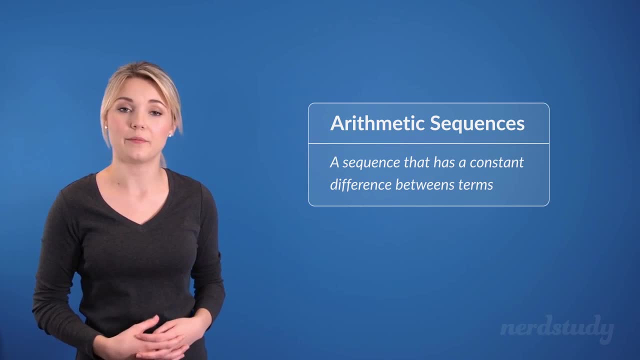 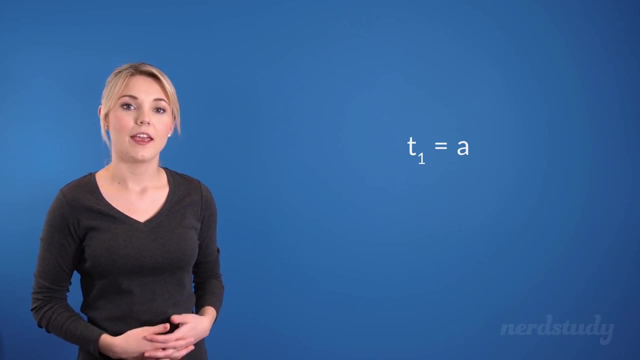 the formula is structured in a way that would look linear in nature, So an arithmetic sequence would start with a number. Let's refer to this number as a for now In that case, since there is a set amount of difference that is always being added on whether that number 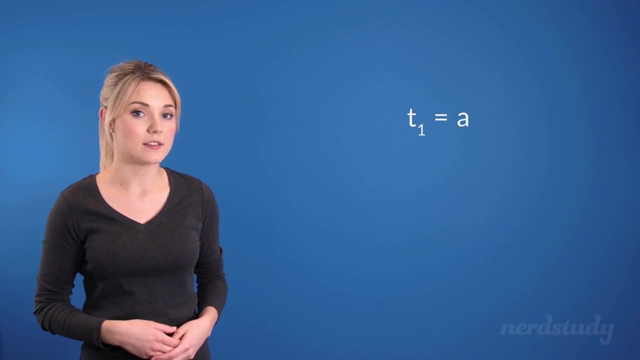 is negative or positive, we can refer to the difference as the common difference, and we'll denote it as d. This means that our second term would clearly be a plus d. Now, from here, our third term would be a plus d. We're going to refer to this as a number. So in this case, 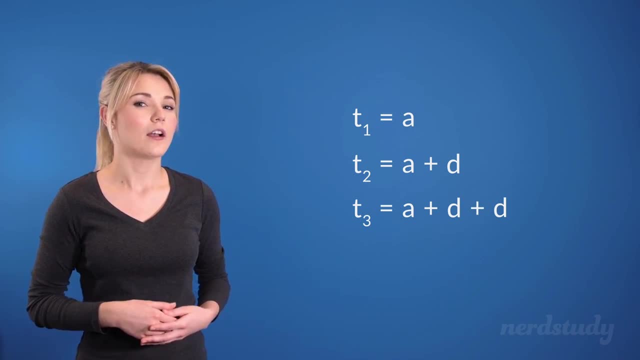 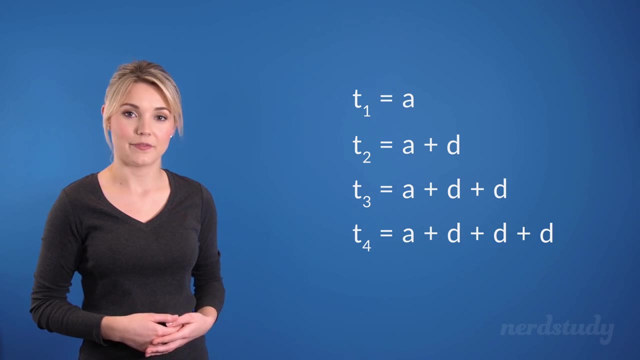 be a plus d, plus d, wouldn't it? And our fourth would just be an addition of d, one more time, giving us a plus d, plus d, plus d. And notice that we can actually simplify this. This here can be simplified to a plus 2d, and this can be simplified down to a plus 3d. But if we look at 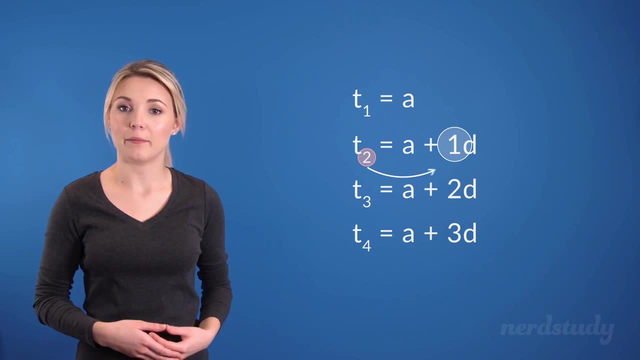 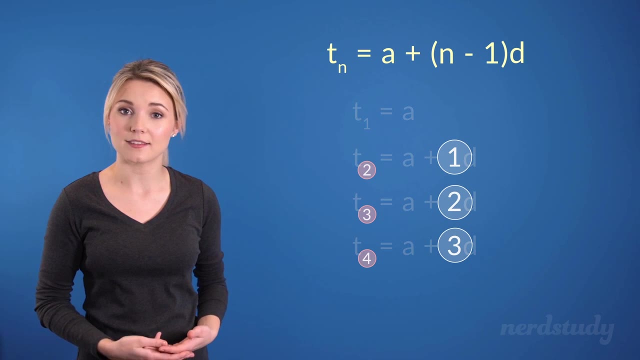 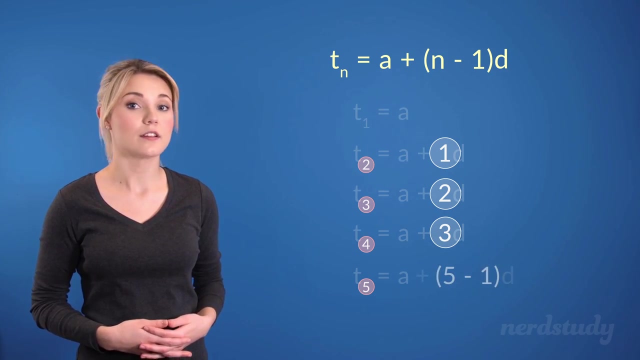 this number here it seems to always be trailing behind by one from what term number we're on. This is easy to account for. however, since we can just write a formula like this, Notice that if we're to look for term 5, then we'd get t of 5 is equal to a plus 5 minus 1d. 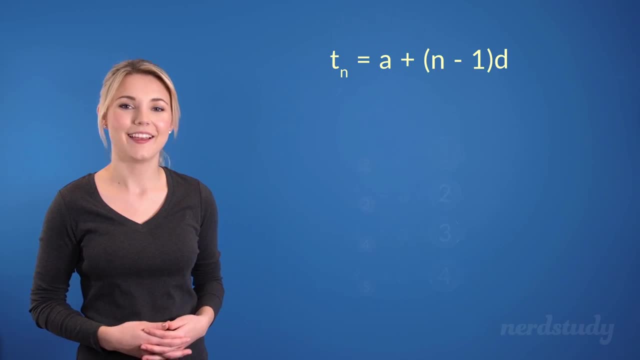 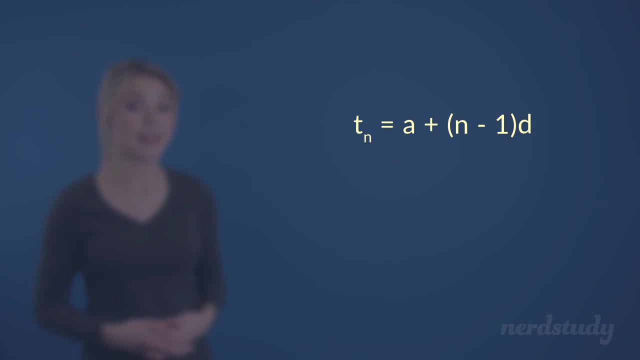 which becomes 4d- Awesome. So let's put our newfound formula to the test and try an example with some numbers. If we had a sequence like this, we would first realize that our first term is 4, which is the a in the formula. 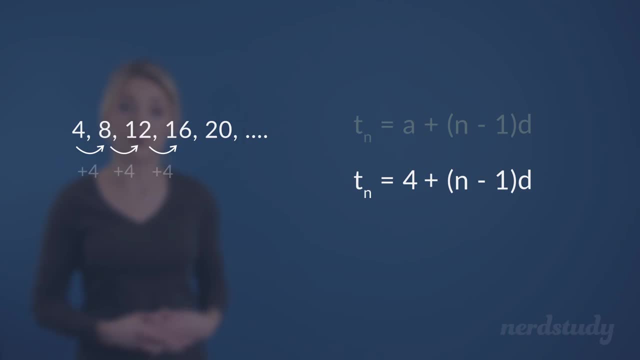 Then we would realize that the difference between each term is also 4, making that our common difference, which is represented as d in this formula. Thus, this would be our formula created for this sequence. So if we wanted to solve for the sixth term, all we would have to do is plug 6.